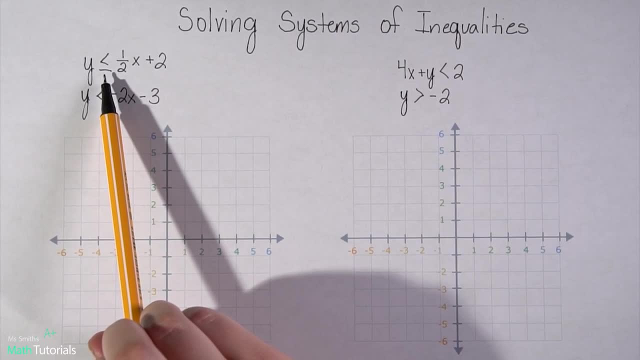 equation: Y equals. now I know that's not an equals, it's an inequality, but we're going to treat it as an equals. So y equals mx plus b. So yes, that first equation is definitely in slope-intercept form. 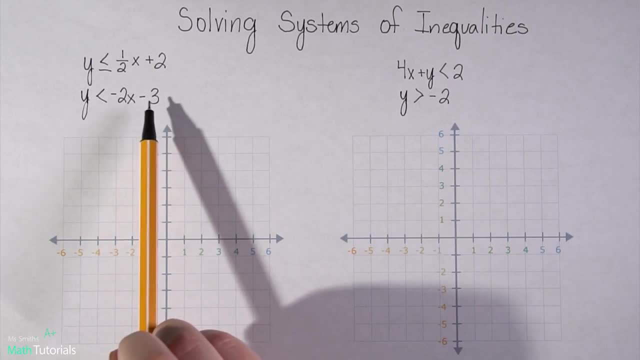 Let's look at the second one. Y equals mx plus b, Yep for sure. So it's okay that this is minus and I'm saying plus. that doesn't matter, As long as it's in the right form and everything's in its 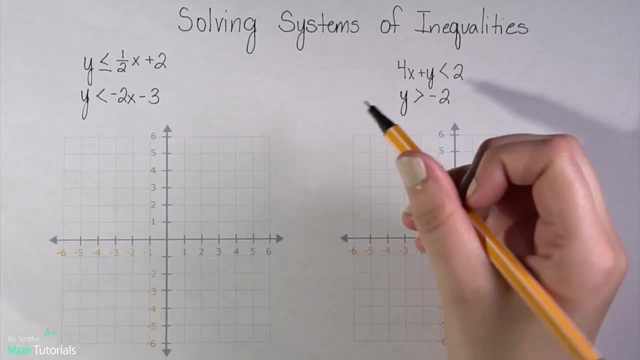 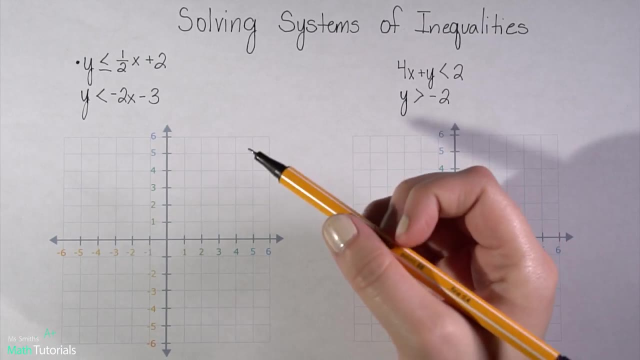 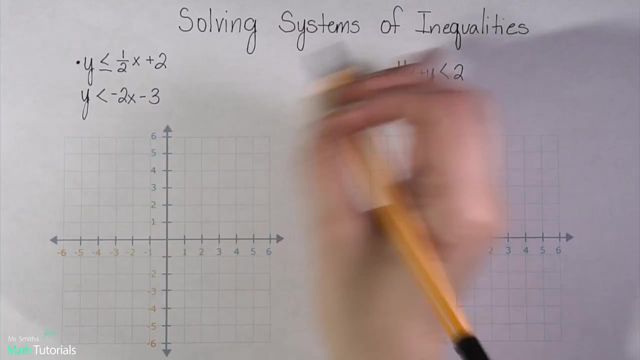 correct form So I can go ahead and graph them. So let's graph this first line. I'm going to do it in black Graphing the exact same way as we would a regular equation. I'm going to plot my first point at my b value, So my y-intercept is at positive two. So here I go. One, two, That's my 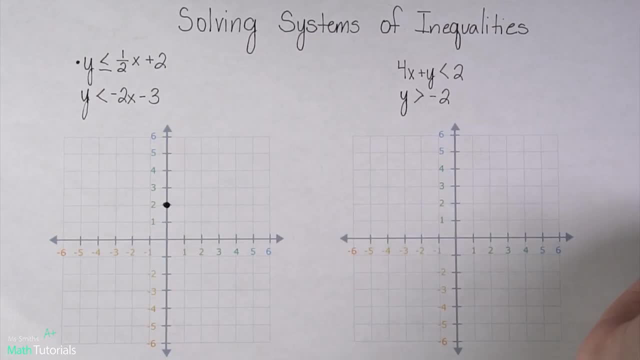 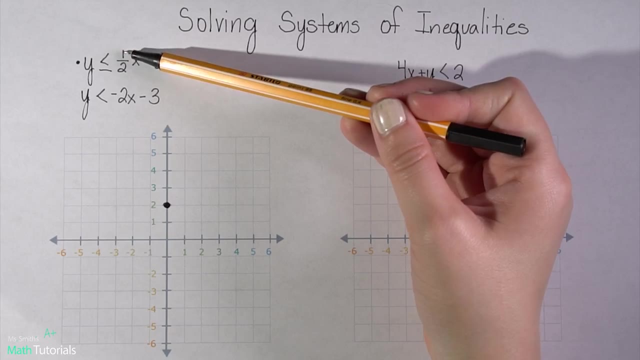 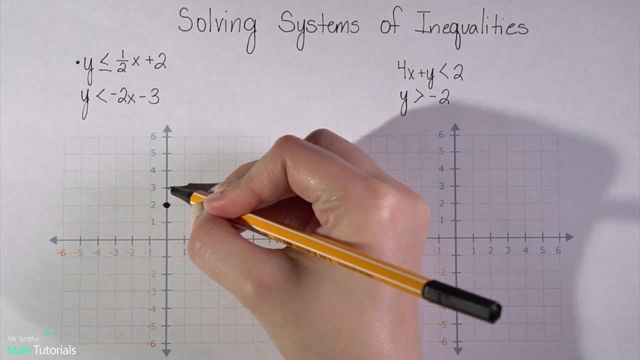 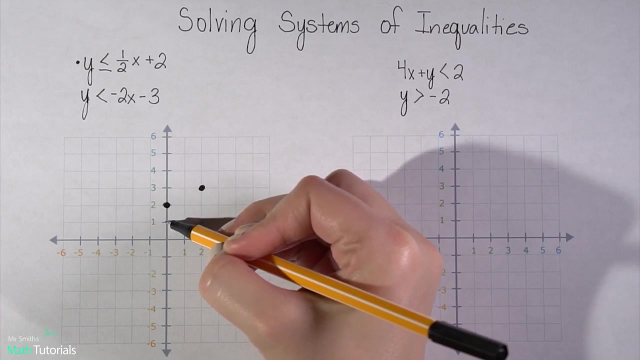 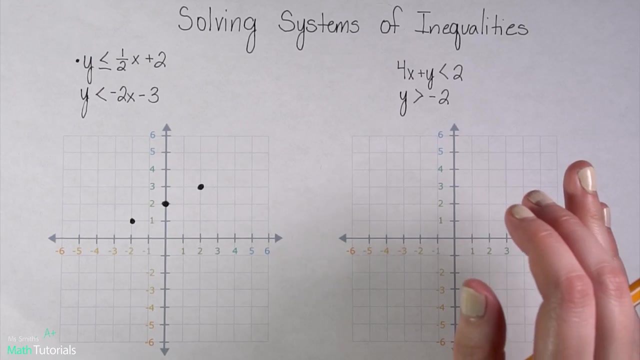 y-intercept point. From there I'm going to move based on what my slope tells me. So my slope is positive one half. So that means that I'm going to be moving up one right, two And I can also do the reverse Down one left, two- And notice it falls all on the same line. Now, before I connect, 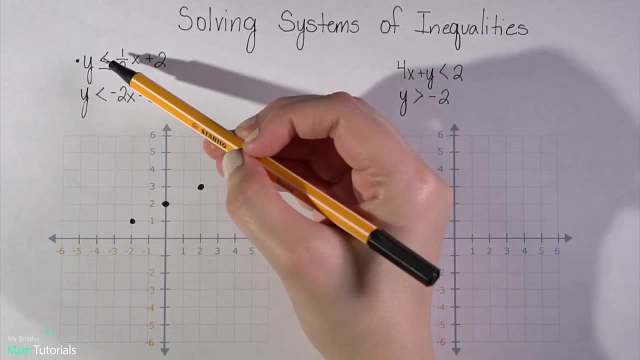 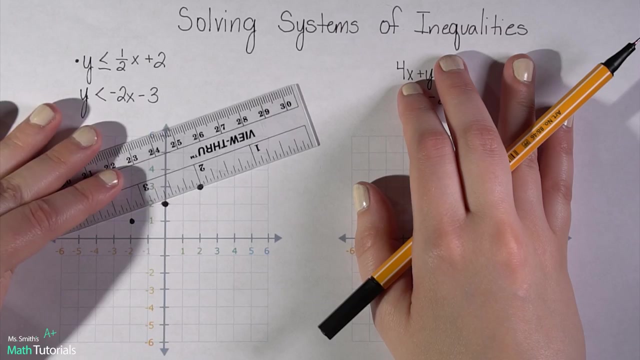 these dots. I need to be real careful and notice: is this a just a less than, or is it a less than or equal to? And in this case it is a less than or equal to. So if you think back to that graphing inequalities video, that means I'm going to be using a solid line. 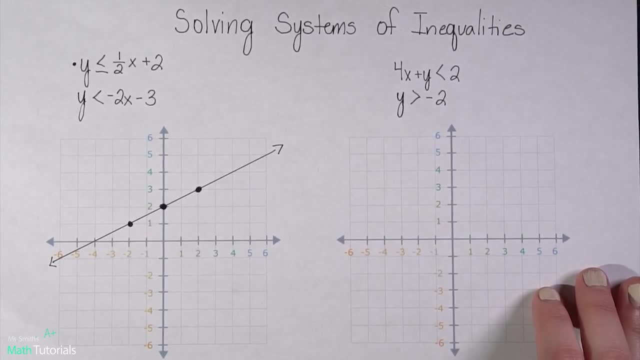 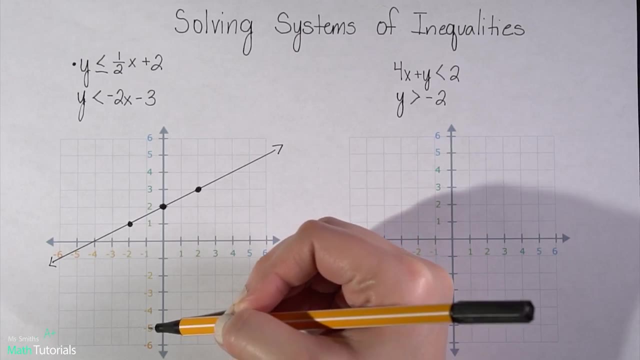 Okay, And because it is a less than, that means I'm going to be shading everything below the line. So if it's ever tricky for you to think, okay, what's the best way to do this? I'm going to be shading everything below the line. 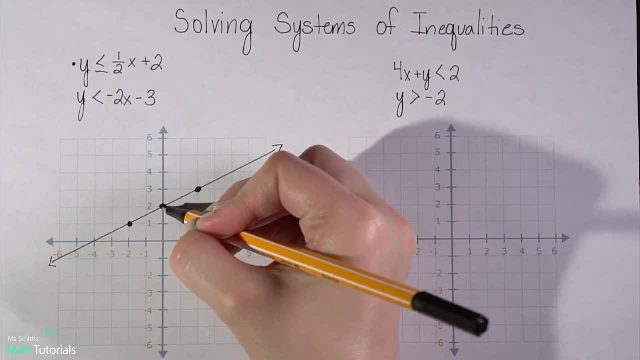 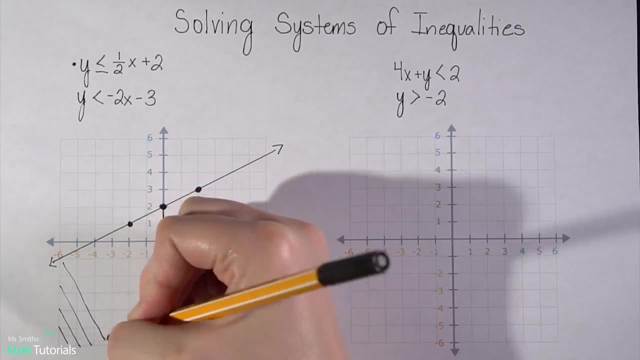 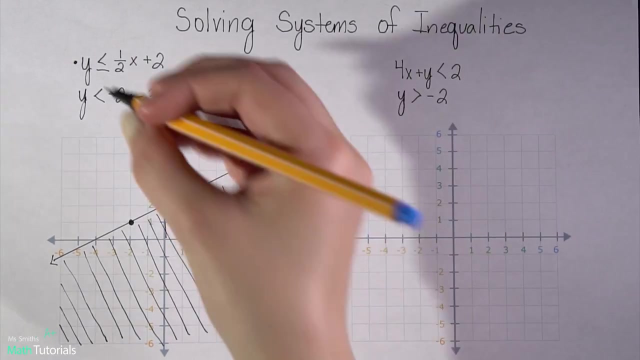 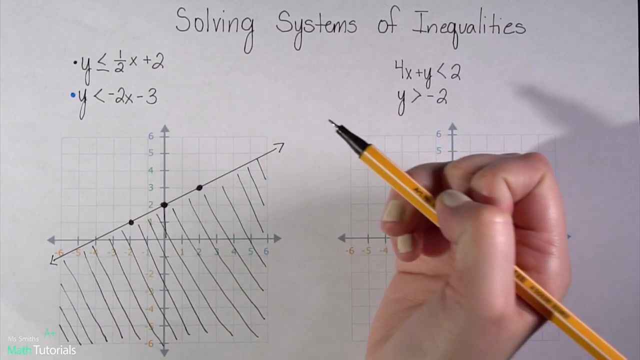 What's below and what's above. Just put your pen on a dot and then pull down. Okay, That whole area is what you're going to shade. So I'm going to shade in black. I'm going to plot the second line in blue. All right, So plotting the same way. I see that my y-intercept is negative. three: 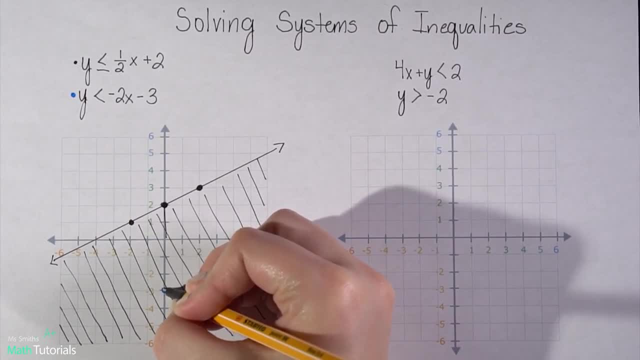 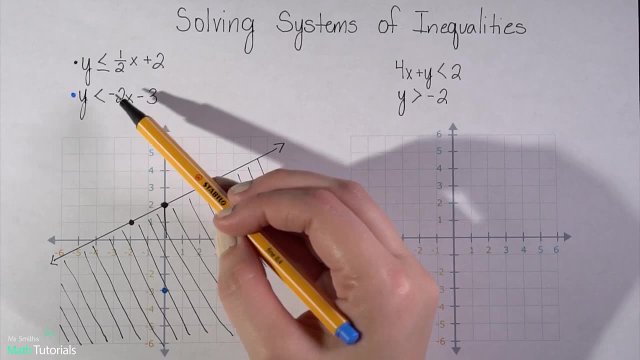 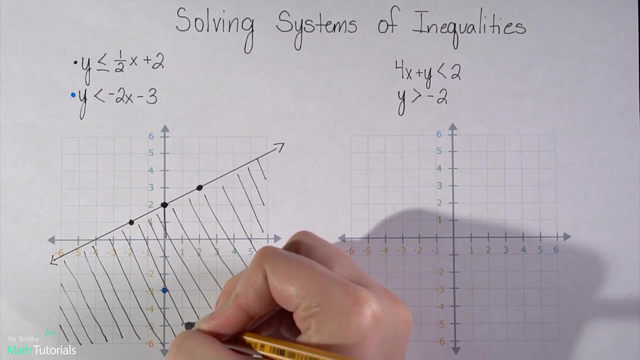 So I'm going to move down three from the origin. That's my first point, And from there my slope is going to tell me how to move. So this is negative two over positive one. So that means I'm going to move down two over one. 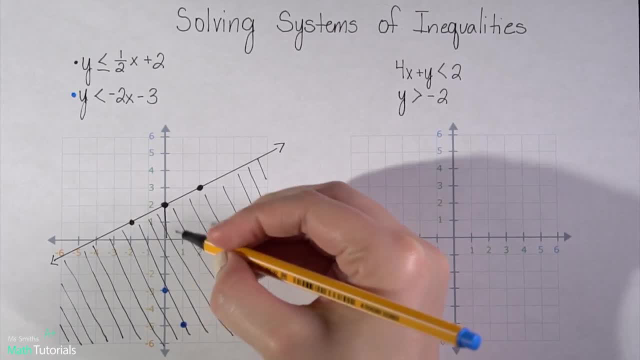 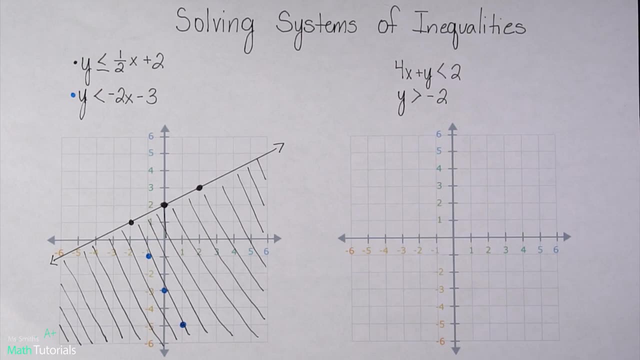 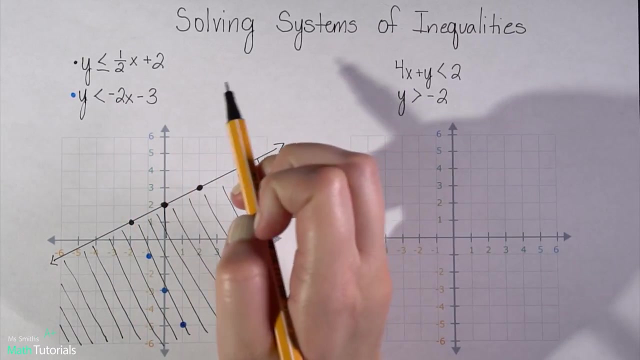 And I can also do the reverse. I can move up to left one. So now let's connect these dots. Now you'll notice that this is just a simple less than. It is not a less than or equal to, So I'm. 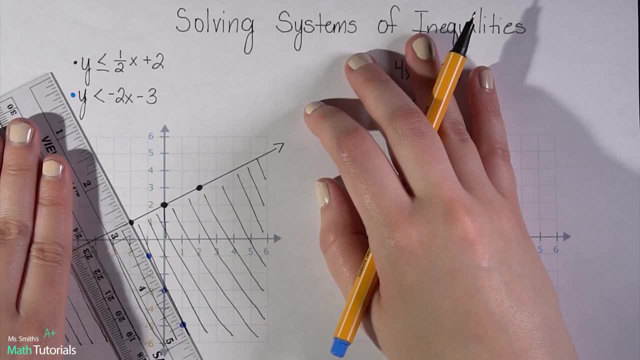 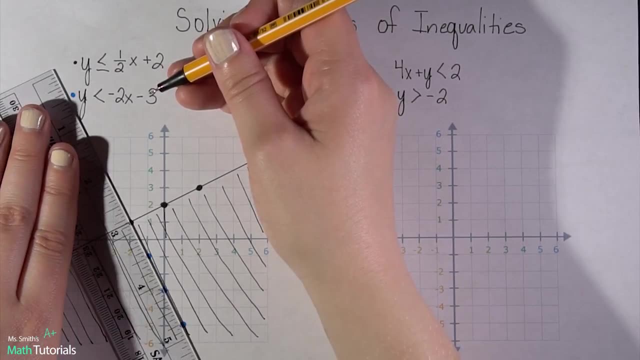 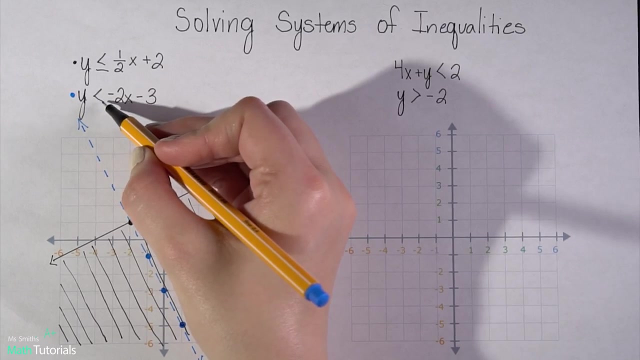 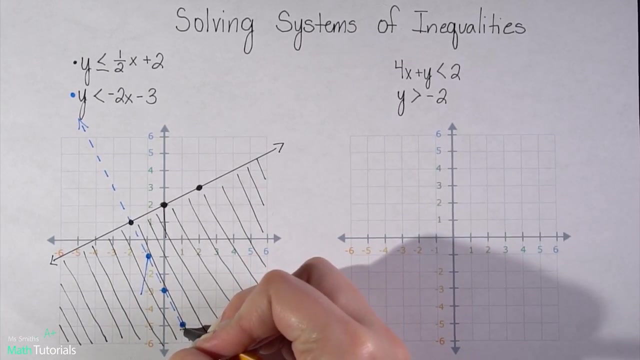 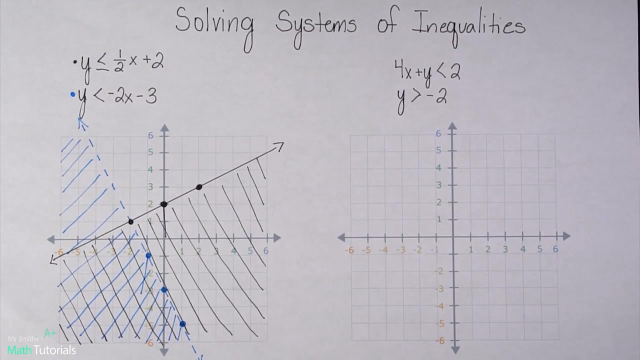 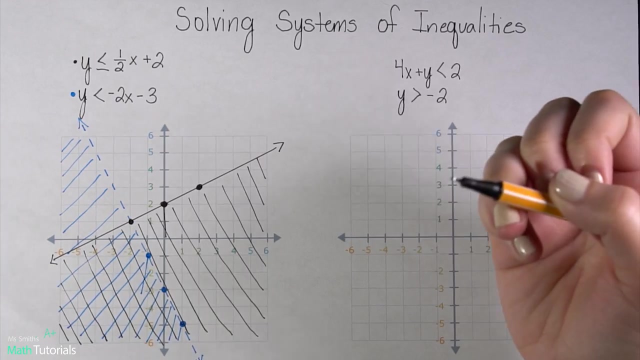 actually going to have a dotted line in this case, Okay, And since it is a less than, I'm going to put my pen on a dot and move Down, So everything below that line is going to get shaded. So, looking at this, at what I've created here with this graph, I'm looking for whatever overlaps. 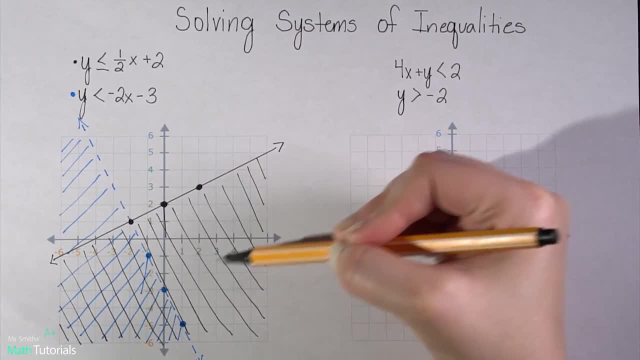 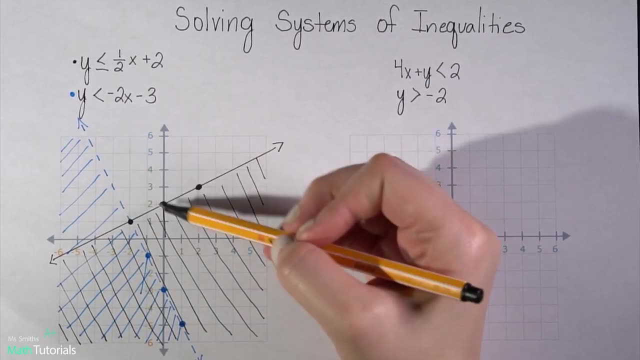 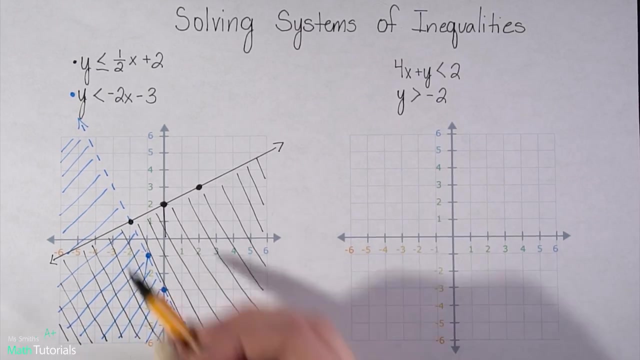 So I'll notice. this area right here is only shaded in black. This area up here is only shaded in blue. This area is not shaded at all, But this corner area right here, it's shaded in black and blue. So this right here, this section, is going to be my solution, So I could pick. 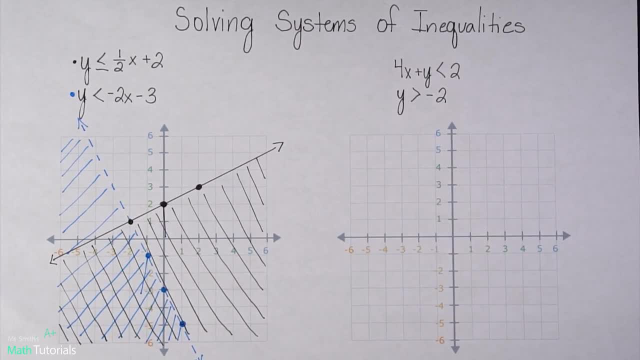 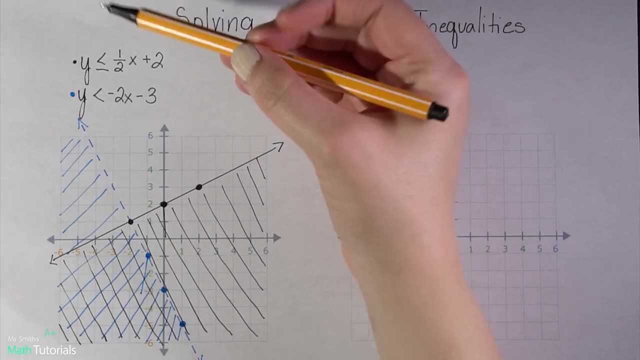 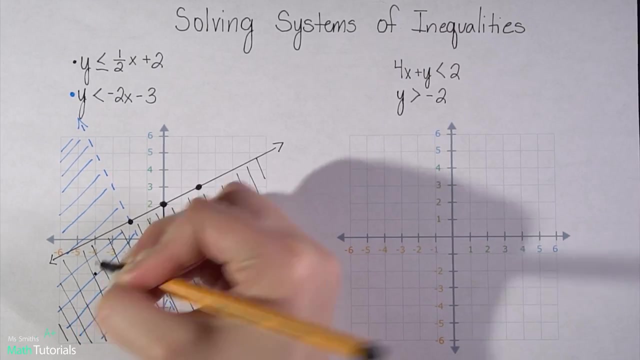 any point within that section, as well as extended beyond the graph. what would fall in that section? Anything I choose would be a solution that would make these statements true. So, for example, I could pick this point right here: All right, That negative four, negative two, Because it falls. 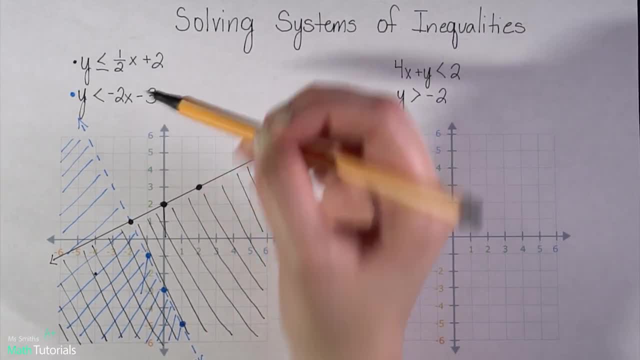 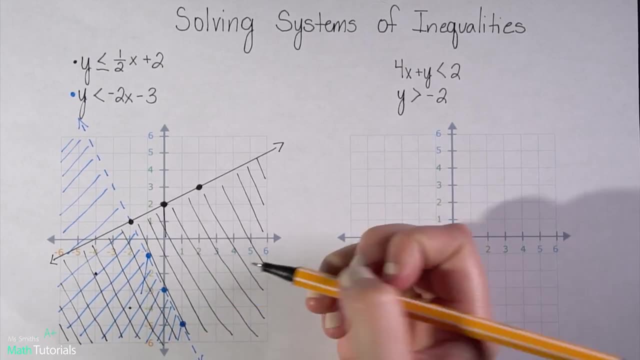 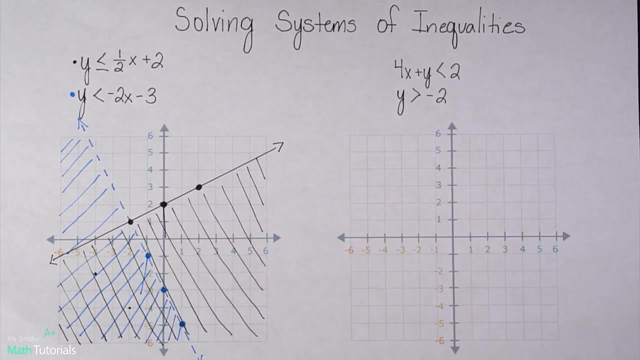 within the shaded region. that would be a true statement for those inequalities. I could pick a different point. I could do this: one Negative, two negative four. Oh, I just did the reverse. That's funny, Doesn't matter. Okay, As long as it falls within that shaded region, it would be a 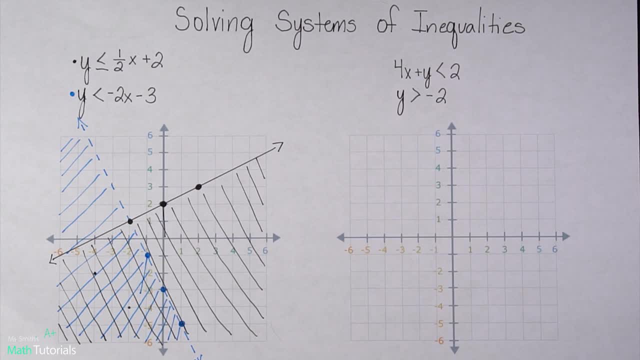 solution to those two Inequalities. So let's look at our second example. So my first equation. I definitely see this is not in slope-intercept form, It's not in y equals mx plus b form, So I've got to get it in that form. 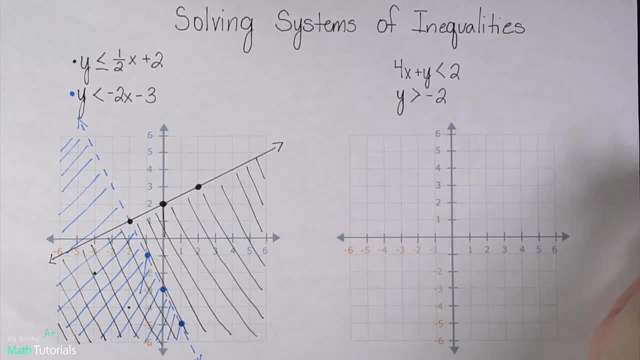 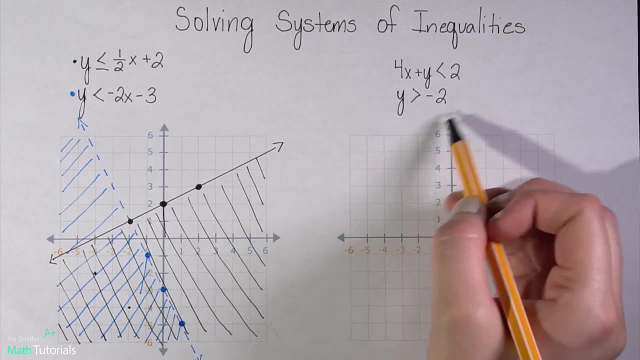 My second equation. yeah, it is in y equals mx plus b form. There's not as much information, but it tells me everything I need to know. I can graph that line, So let's get that first one in the right form. So four negative, two negative, three negative, four negative, three negative four. 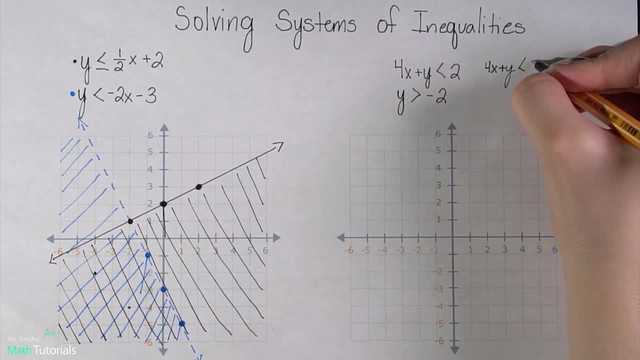 negative four negative three negative four negative three negative four negative four negative four negative three negative four positive four negative four negative three negative four negative four negative three negative four negative three. I would want to get my y alone. 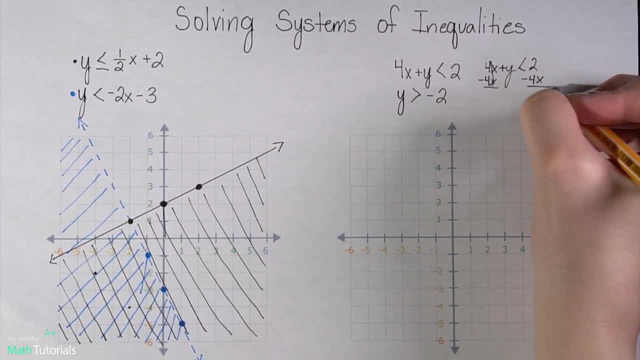 So I'm going to move this four x over. I would have: y is less than Now. I can't combine 2 minus 4x, but I can rewrite them in standard form, keeping their signs. So the negative stays with the 4x, the positive stays with the 2.. Now I've 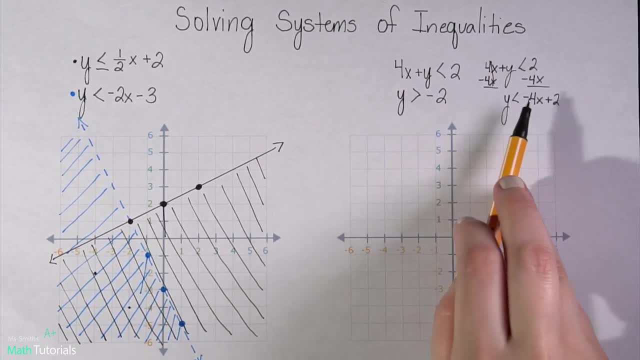 got an equation in slope-intercept because it changes the killed rheumatism. So you need negative two in slope-intercept form that I can graph. So let's do this one first in black and then we'll come back and do that one. 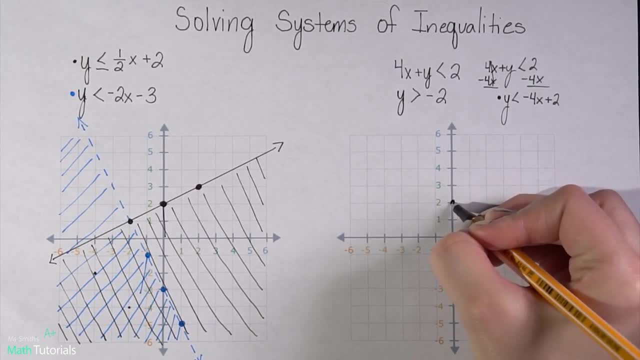 So I'm going to plot my first point at that: positive 2, right there, And from there it says: I want to move down 4.. This is negative, 4 over positive, 1.. So down 4, 1, 2, 3, 4, over 1.. 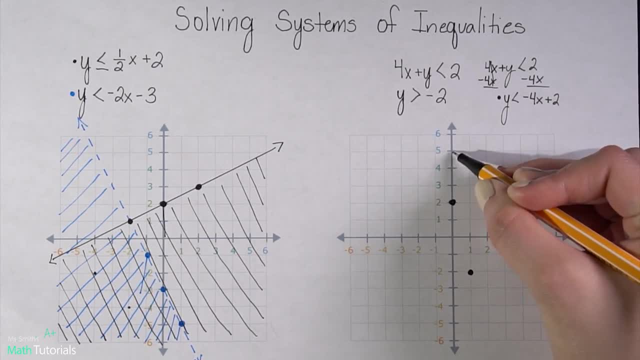 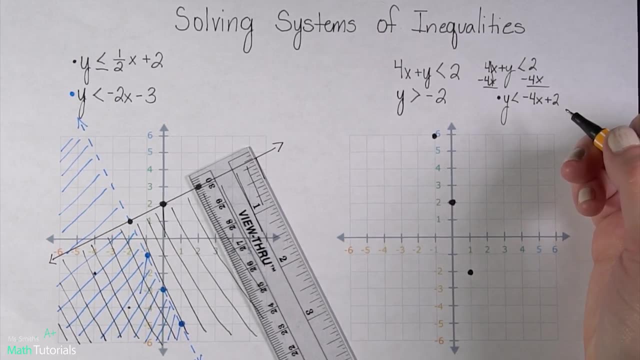 And you could do the reverse. I could move up 4, 1,, 2,, 3, 4, left, 1.. All right, let's connect that line. You'll notice that this is a less than, not less than or equal to. 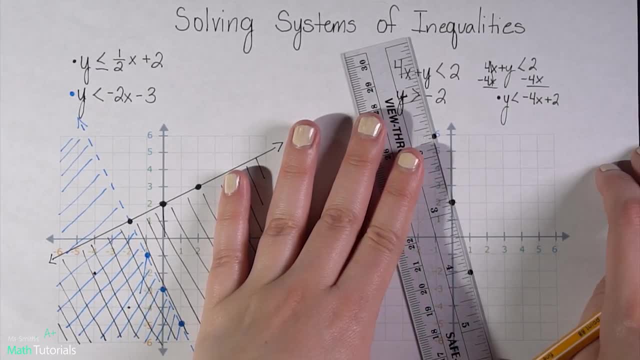 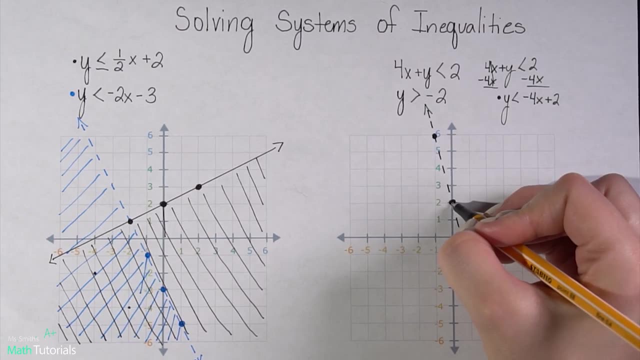 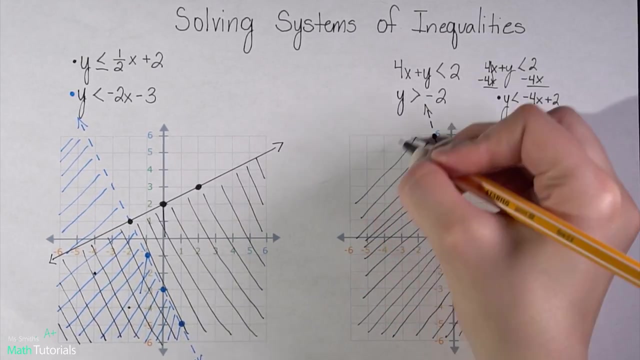 So it's going to be a dotted line, All right, and because it is less than I'm going to shade below, So I'm going to put my pen on one of my dots and move below. Everything below will get shaded in black.